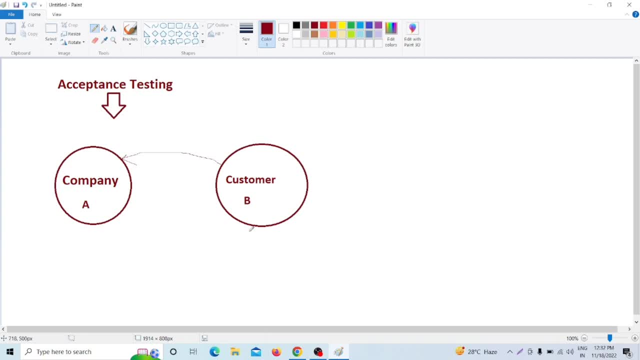 why what we'll do then the customer. that means the customer is requested. what is happened? the customer is requested to make any software, so that's why what we'll do then the customer that make the software to make the software okay. so that's why software. so that's why the customer. 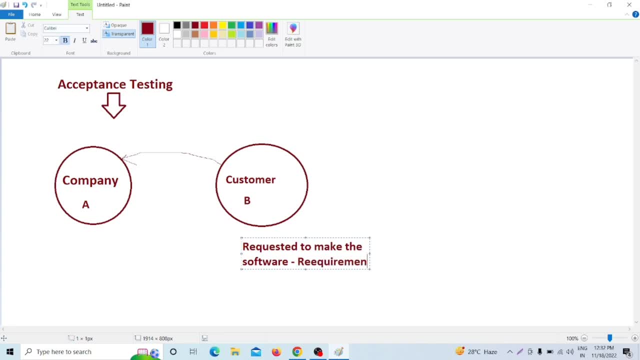 B has given some requirement requirement. the company: okay, so requirement, now requirement. so that's why the customer B requested to make a software to the company A. that's why the customer B has given some setup requirement. the company: okay, now, what we'll do now, company will take that requirement from the customer. what we'll do, company will take that requirement from. 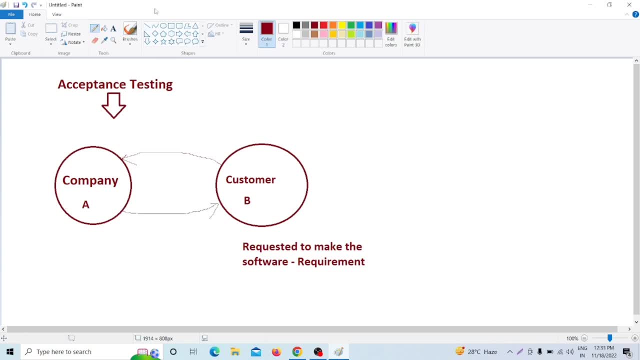 the customer and, as per the requirement, the company will making the software. will that means company is making the software okay. so that is the main, main thing. so customer has given some requirement, requirement and the customer will give the requirement to the company and, as per the requirement, the company will making the software. 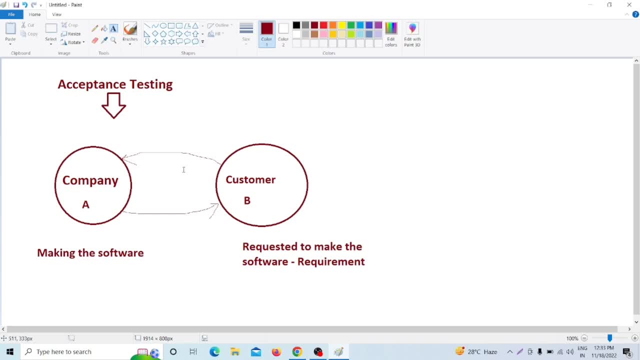 okay now, let's say, the customer given some set of period period of time, let's say customer has given some set of period, the company A will make the software and he will hand over that fully make software to the customer. okay, so that is the main thing. okay, so whenever the company A will complete the software, then what he will do, he will do the do the software to the customer B. okay, now here the acceptance testing is coming to the picture. so whenever the company A will complete the software, then what he will do, he will do the do the software to the customer B. okay, now here the acceptance testing is coming to the picture. so whenever the company A will complete the software, then what he will do, he will do the do the software to the customer B. okay, now here the acceptance testing is coming to the picture. so whenever the company A will complete the software, then what he will do, he will do the do the software to the customer B. okay, now here the acceptance testing is coming to the picture. so whenever the company A will complete the software, then what he will do, he will do he will do the do the software to the customer B. okay, now here the acceptance testing is coming to the picture, so whenever the company A will complete the software. 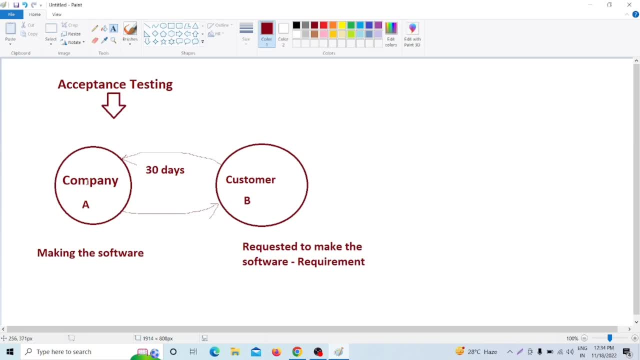 the customer is taking that software to the company a, then what testing will be done by the customer? that is called the acceptance testing. customer will tell the company, yes, after testing the software. they will respond that company a that yes, i am accept your software, that, whatever you build, that is the acceptance testing. ok, so in a simple word, 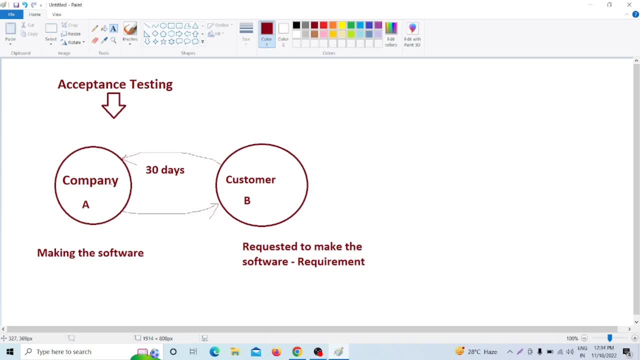 in a simple word what we can say. we can say that acceptance testing is a type of testing that is performed by the end user or the client to verify or accept the software system. before moving the software application to the production engine environment, before going to the live, the customer will test the software that is called 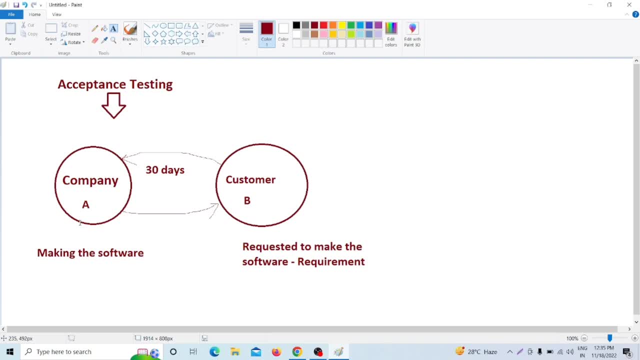 the acceptance testing. the customer can test, the client can test, ok, so that is called the acceptance testing. so acceptance testing is a end to end testing, end to end testing. so now, guys, you have a very much. you have a questions in your mind that what is end to end testing? 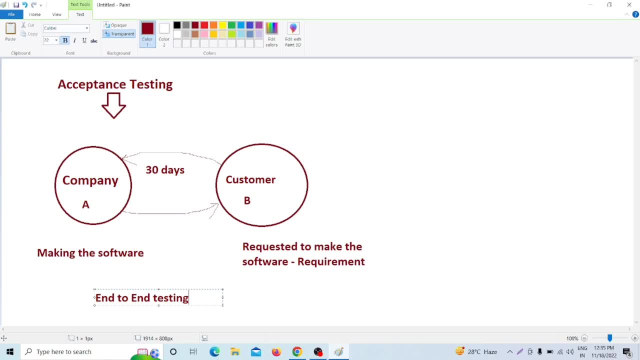 i will tell you what is end to end testing. so now i am telling you that what is acceptance testing? acceptance testing, it is a end to end testing which is given by a customer to a particular period of time to make sure that the software is able to handle with the real. 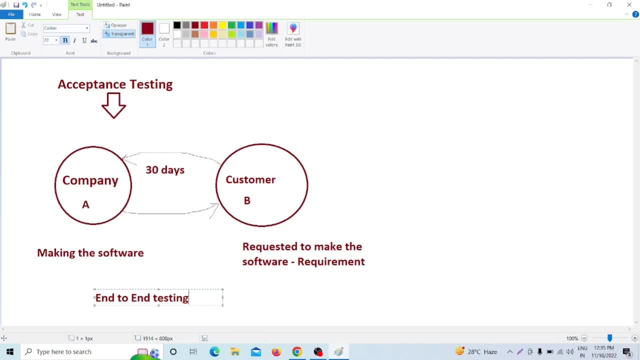 time business scenarios or not. that is called acceptance testing. obviously, when the customer will test the application which is made by the company, obviously the customer will test some set of real time business scenario. ok, that means, what is real time business scenario? let i am giving you one very basic. 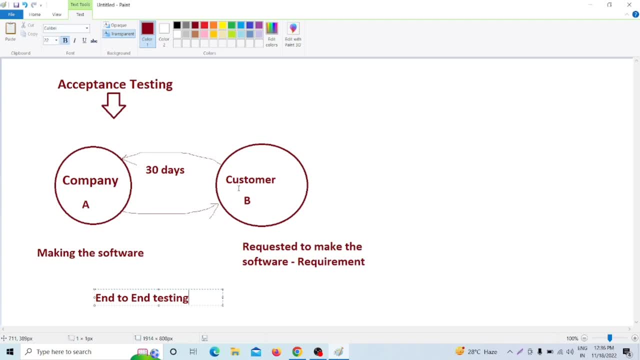 example, that let us say one site that is called flipkart. so what is the flipkart main functionality? that we can add any product. we can purchase any product. so purchasing is the main thing: to buy any product. that is the main fund of flipkart. i suppose i want to buy any mobile. ok, and obviously i will go to the flipkart and i will. 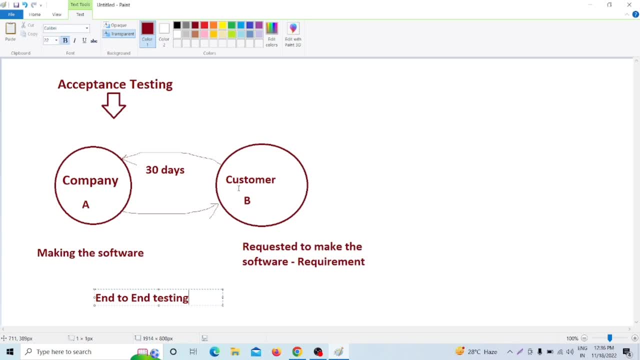 search that particular mobile and i will add that mobile to the to my cart, then i will payment that mobile, i will payment price for that mobile and then i will purchase that mobile. that is the main fund of flipkart, so whenever. so what is the real time business? 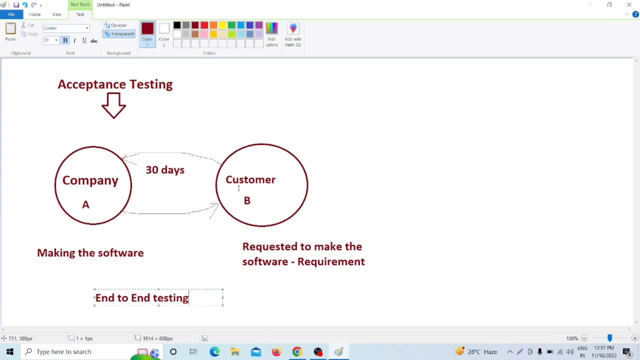 scenario. real time business scenario means in which business scenario, customer can purchase the mobile, they can go forward their business, their software business. that is the real time business scenario. so now, guys, we have very much clear idea about what is acceptance testing. so acceptance testing is a type of software testing. which is performed by whom? which is performed by client or end. 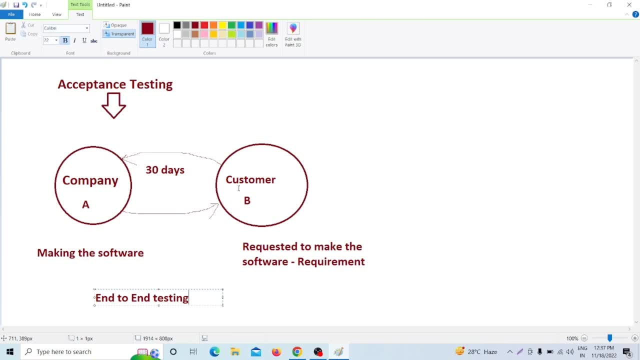 user to verify or to accept the software system before moving the software to the production environment or live environment. that is nothing but called a called an acceptance testing. ok, so acceptance testing is a end to end testing which is given by the customer to a particular period of time to make sure. 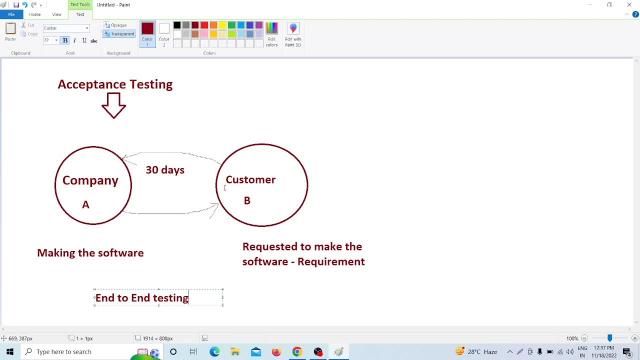 that the software is able to handle with all the real time business scenarios or not. that is called the acceptance testing. that means we are accepting the software. that means customer is accept accepting that software which is made by the company. that is called acceptance testing. now what? 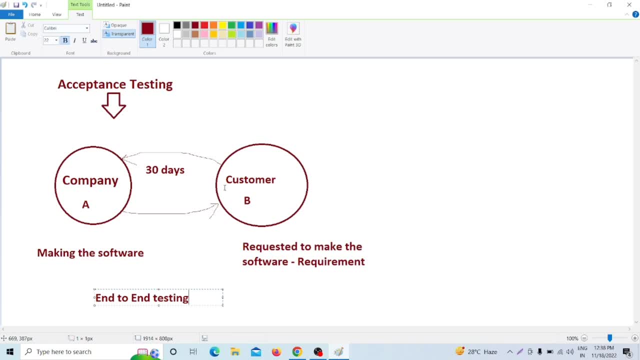 is end to end testing. i have already told you in the definition of acceptance testing that acceptance testing is the end to end testing. so what is end to end testing? so end to end testing. i am giving one example: end to end testing means navigating through all the features and making sure that the end feature or last features of the software is. 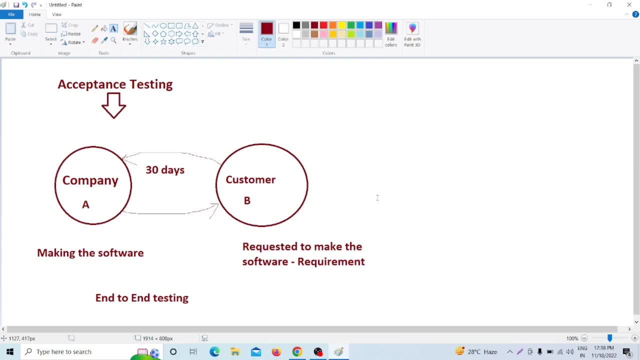 working fine or not navigating through all the features, like suppose, let's say i am. let's say this is one module. ok, this is one module. this is one module. this is one module. let's say there are five module in a application, so just you can assume that it's a flipkart. 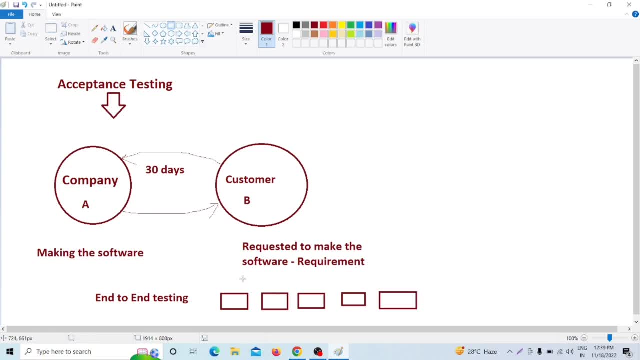 application. so in the flipkart application there is five modules, just for example. let's say one is login, another is search page, then add to cart page, then payment page and then order confirmation page. let's say five, application. so what is what i am telling in end to end? 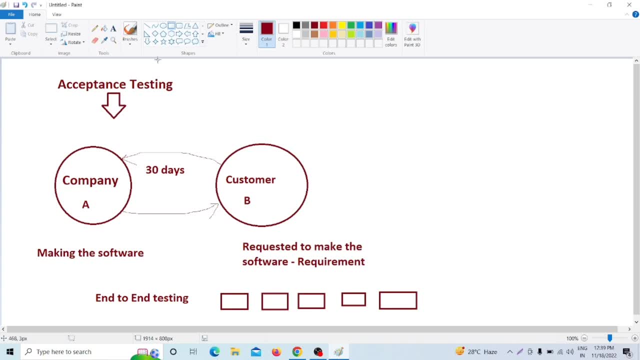 testing that navigating through all the features. so we have to navigate through all the features and make sure, navigating through all the features and make sure that the last features of the software is working fine or not. that's the end to end testing or end features is working perfectly fine or not. that means suppose i have. i i did the login in the. 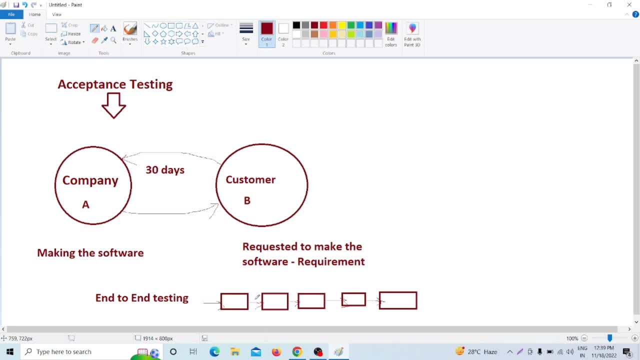 flipkart. so after login, what i will do? login is not the real-time business scenario. so then i have to search any product, then i have to, i have to add to cart that product, then i have to, i have to make payment for that product, and after that i will go for the order confirmation page. so until we are, 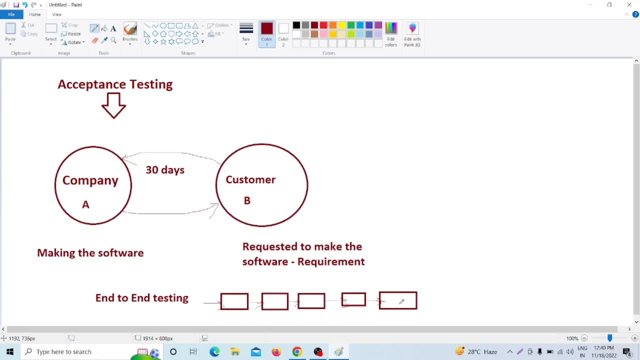 getting the order confirmation page. we cannot do that until let our order is, i mean purchased by the flipkart. we cannot tell. so that means last feature is the final features, where I can tell anyone that, yes, my applications is working perfectly fine. so that is done on the end to end testing that navigating. 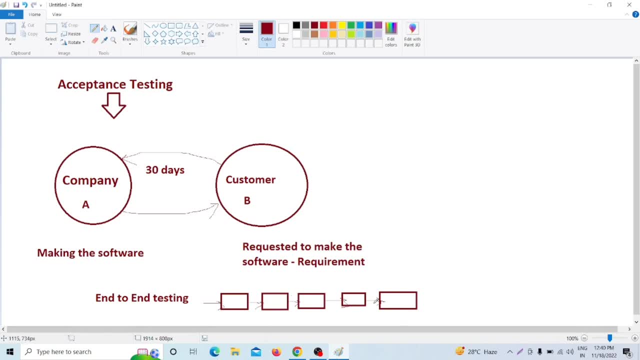 through all the features and the last feature of the applications is perfectly working fine or not. either last features is working perfectly fine, then we can blindly tell this: our application is here, then we can wait here. only at this point. and when I try to update to my application then i am unable to sort it out. 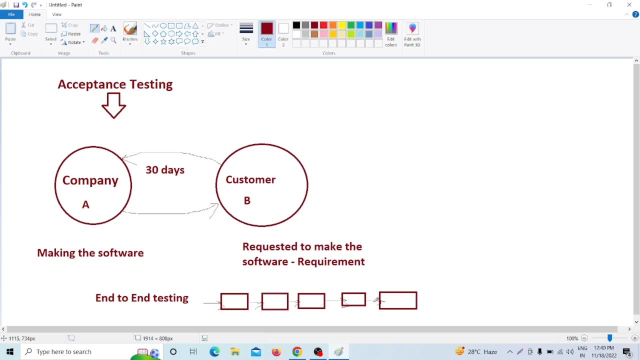 mainly tell that the before functionality- i mean the fourth, number three, number two, number one- all these modules are working perfectly fine. if these features are not working perfectly fine, then obviously we cannot go to the last feature, so as because these modules are working perfectly fine. so that's why i'm the order confirmation page. so that is the end-to-end. 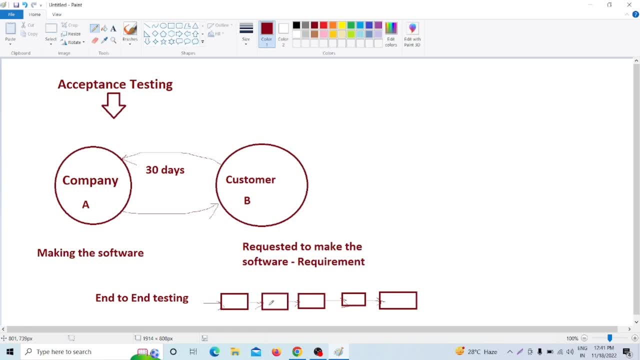 testing means navigating through all the features of an application and make sure that the end features, or the last feature of the applications is working perfectly fine or not. that is called as end-to-end testing. okay, so now you guys are very much clear about that. what is acceptance? 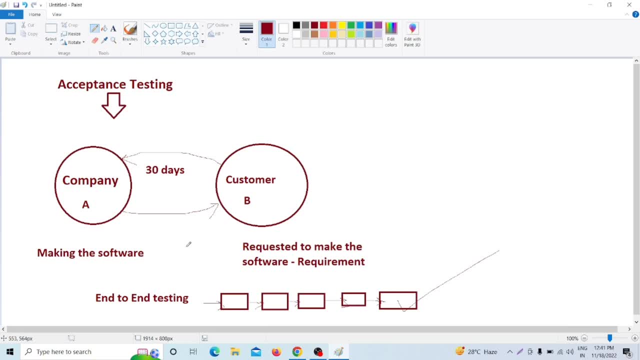 testing. acceptance testing is nothing but a end-to-end testing which is given by the customer for a two applications for a particular period of time, to make sure that the software is able to handle with the real-time business scenarios, or not, right? so who will do the acceptance testing? the? 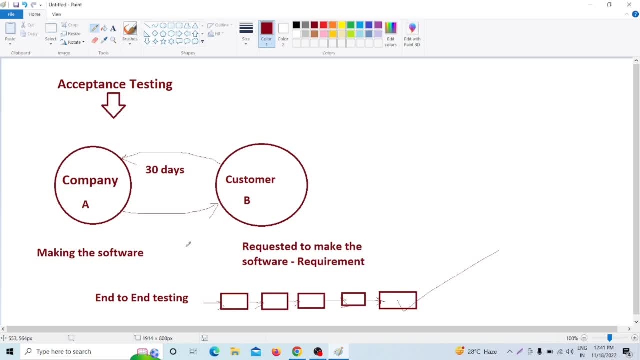 customer or the end user or the client will do the acceptance testing. okay, so now you are. you guys are very much clear about what is acceptance testing. now the next point is that so there is many names for that acceptance testing. we can, in a, in a different, different company, they will, uh, they call the acceptance testing the. 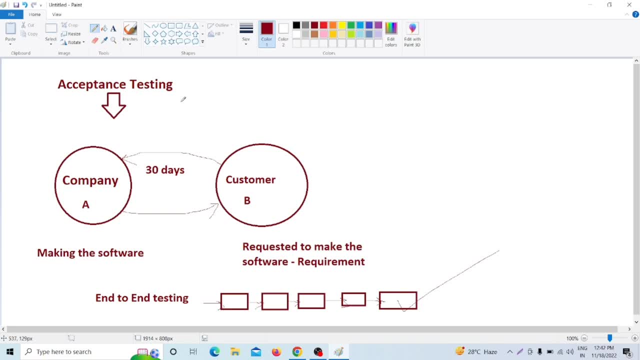 different names. so we can say in a simple word that there are few nickname. is there for that acceptance testing? what is that? what is the nickname? so first we can tell the first name is that uat, uat, that is user, user acceptance testing, acceptance testing, acceptance testing. 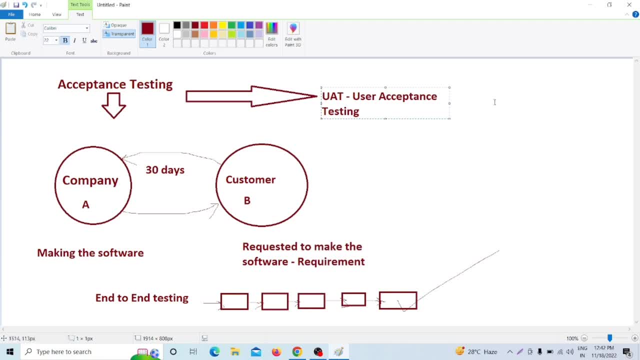 testing, user acceptance testing- okay, so we can tell acceptance testing as the uat or user acceptance testing. then second one: we can tell that fat, fat. or you can tell that final acceptance testing, okay, or we can tell it as like a rbt, rbt, red box testing, red box testing, red box. 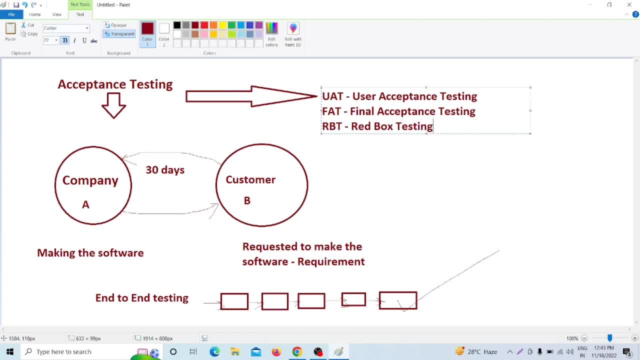 testing or we can tell it as acceptance testing. so acceptance testing. this is the nickname. different different company can use that name name, like your t fat rbt. so in case of your time, if any interviewer is asking you that what is rbt or what is red box testing, so you can tell that. 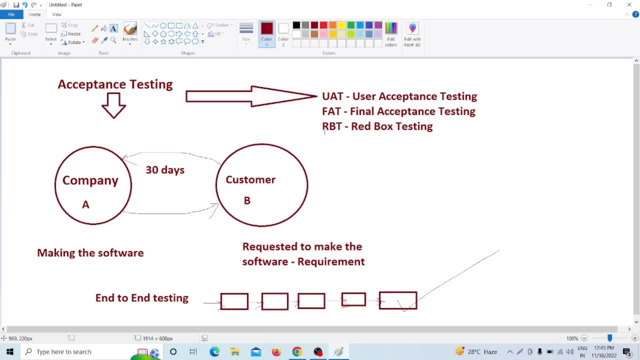 what is acceptance testing okay? or if any companies can ask you that what is user acceptance testing? so you can directly tell that. or you can blindly tell that: what is acceptance testing? that, what i am already to that: what is acceptance testing okay? so acceptance testing is the last stage of 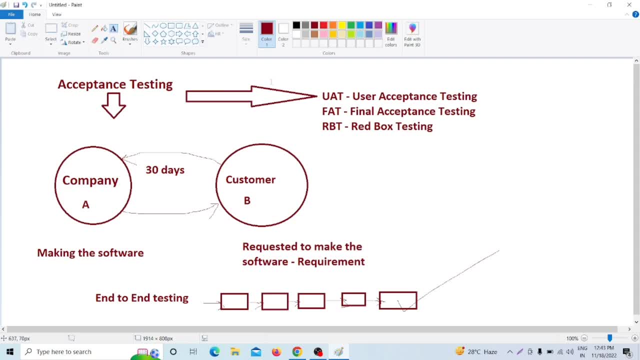 testing. before giving the software to the customer, you have to do the acceptance testing. or before going to the products and environment, the last is that acceptance testing. okay, so now you guys are very much clear about what is acceptance testing now. so i have told you that we have to check the real-time business scenario, right? so what do you mean by real-time? 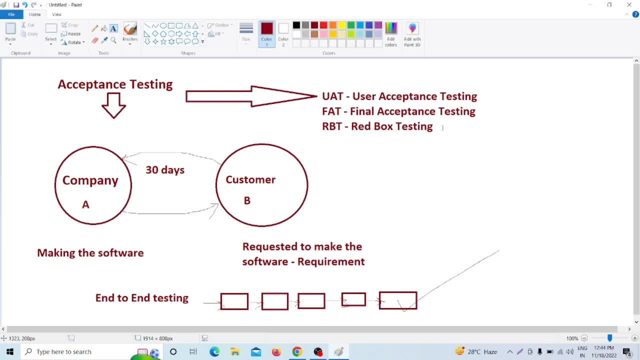 business scenario. i already told you that what is real-time business scenario? so how many ways then customer can do the acceptance testing? what are the ways? are there? so there are few ways. that is totally dependent on the acceptance testing. so how many ways can the customer do the acceptance? 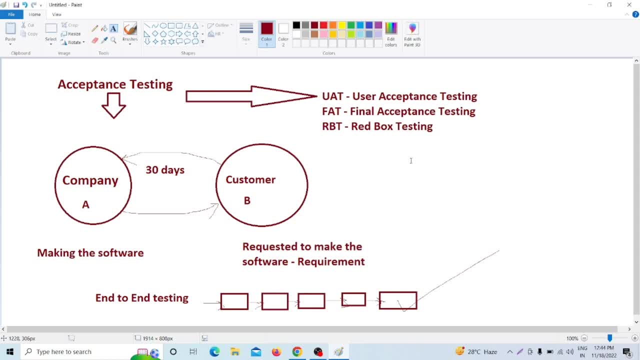 testing on your views. so, as per my view, suppose i can tell you the three or four. as per your view, you can tell more than four, five, six, like that. okay, so it's totally depending upon on your views. okay, so how many ways the customer can do acceptance testing. so i can tell you almost three. 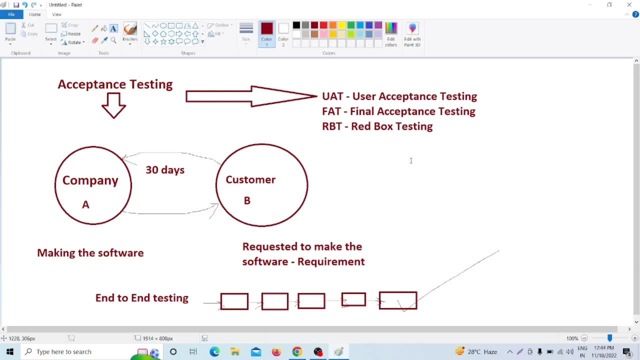 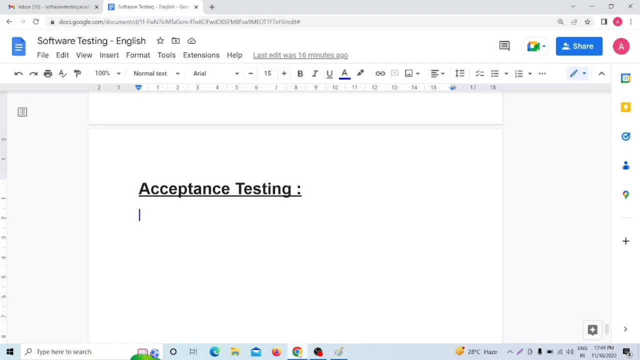 to four views, like four ways. like first, acceptance testing: we have to go for the real-time business scenario. So I can tell you that, what is the ways, ways for acceptance testing, What is the ways for acceptance testing? I can tell you. the first one is that real time business scenario. real time business scenario. 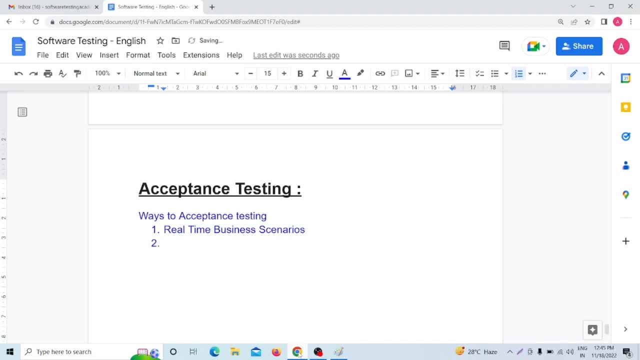 Real time business scenario. What is that? I have already told you that. what is real time business scenario? Real time business scenario means: suppose we are. we are, we are giving some valid input, We are giving some live input. Okay, So, as if, as as of take the application, take the example of a flip card. 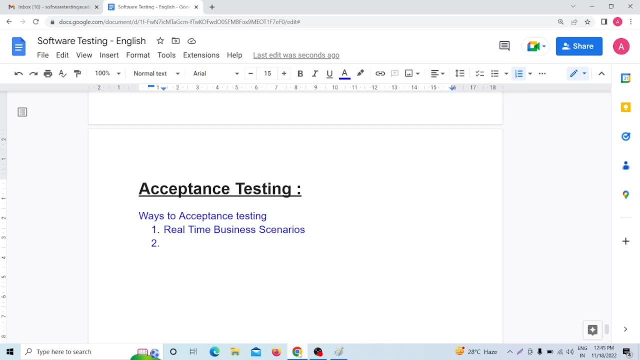 So what is the flip card real time business scenario? So any user can purchase any product from the site, Right? So that is the real time business scenario and the whole flip card is standing up on that real time business scenario. So For the acceptance testing, how many tools are there for one? is that real time business scenario? 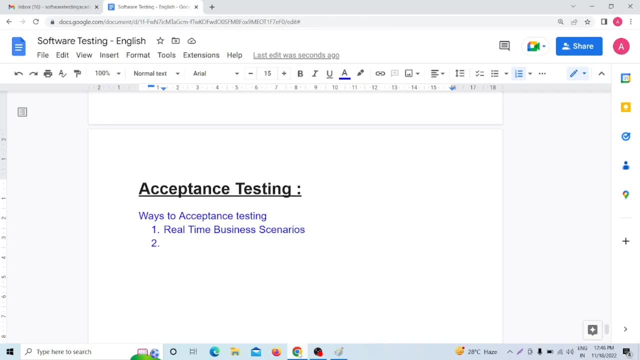 Now, second was that set of real time business scenario. for we can say that, let's say set of real time business scenario, But there is, you can say that set of- I'm giving you the example for that set of real time, Set of real time business scenarios. 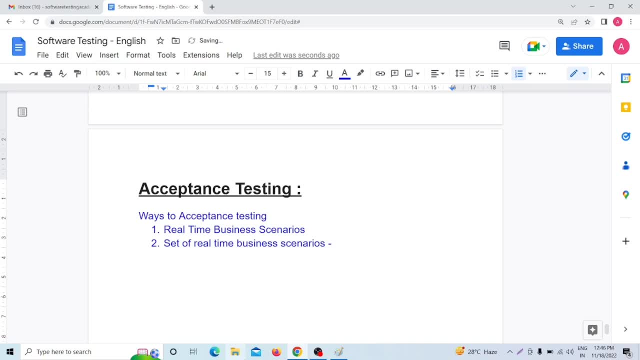 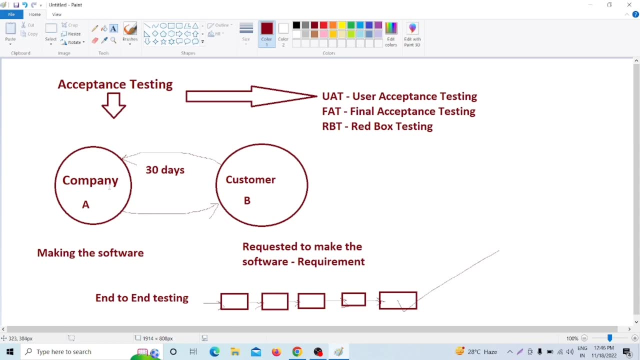 That is depending upon customer or client. customer or company. Let's say, Suppose Take that, take that application. So what is done in that application? So what is in that done in that scenario? Company has completed their software. They are making the software as per the customer requirement. 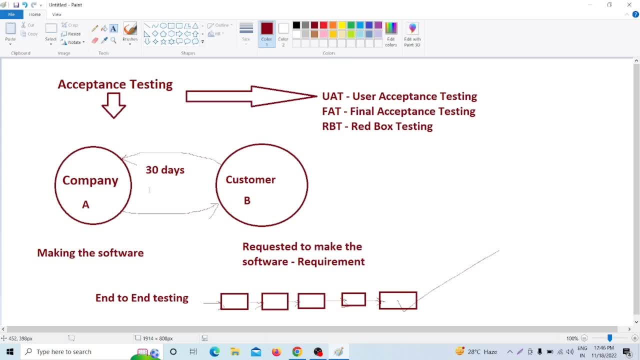 Okay, As per the customer requirement Now set of real scenario, that is done from the customer end. Suppose the company completed the software and he has, he has given the software to the customer. Now, in that customer end, the customer, there is many people are there, like IT engineer, like agent, like some customer. 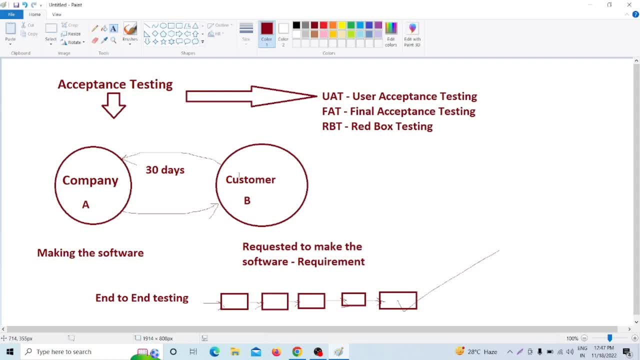 They are present in that, some business analyst, They are in that customer field, So That people will test that application by some real time, Some real time business scenarios. So that is the one thing. Okay, So that is the one thing. 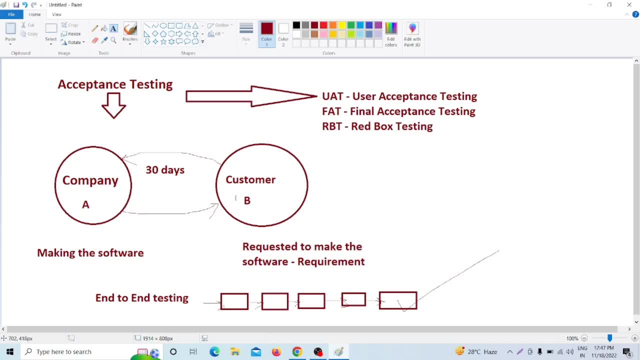 So one thing is done on the customer place. So real time business scenario can be done on the customer place or from the company. any project manager or any business analyst, They can directly fly to that customer place and the customer will give some set of real time business scenario and they will test that application. 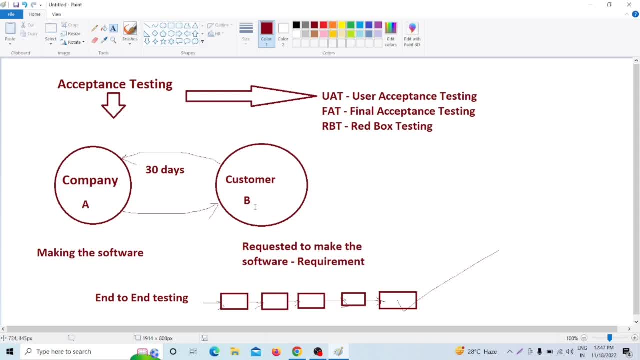 I mean Our business analyst will test that applications by the given some set of real time business scenario by the customer. That is one thing And the another thing is that that from that customer end, from the customer edge, and some BA, some IT engineer or some agents are there. 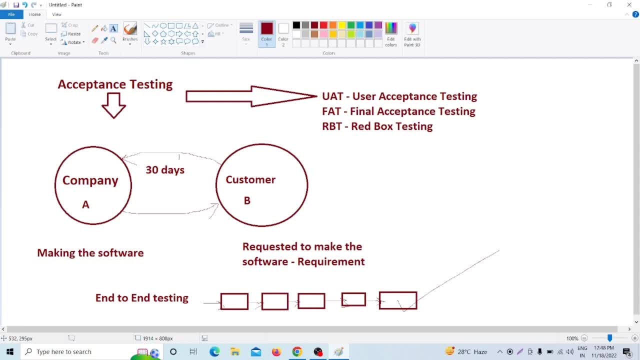 So they can directly fly to that customer, that company place, or they can directly go to the company place and then with some set of requirement, So in that, let's say in that customer place, some people are there like IT engineer, like IT engineer, like IT engineer, or I can say BA or I can say agent. 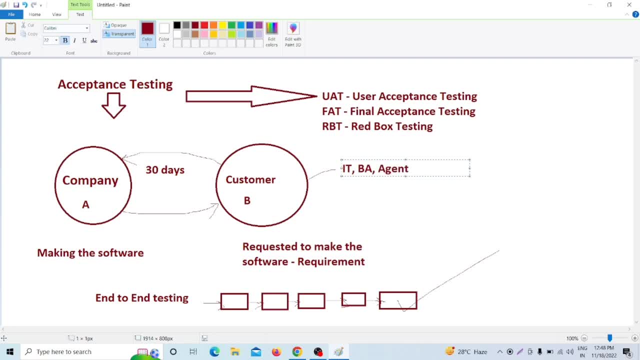 Some people are there. Okay, Some people are there. So they will directly go to the company's place with some set of requirements by their hand And then they will ask someone from that company or some tester from that company end That I have set up. 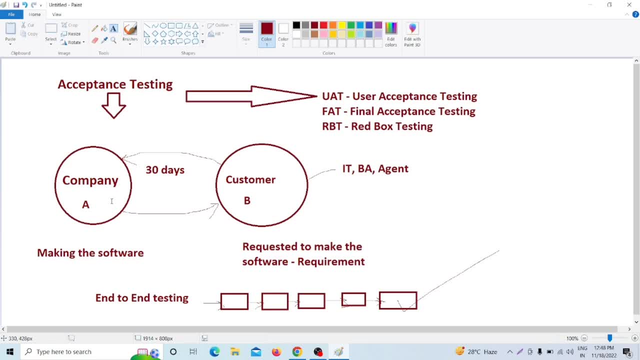 I have set of requirements in my hand So you guys can please check on it with the real time business scenario that your application is working perfectly fine or not. Then what we'll do Then the, then the company's tester or company's any employee. 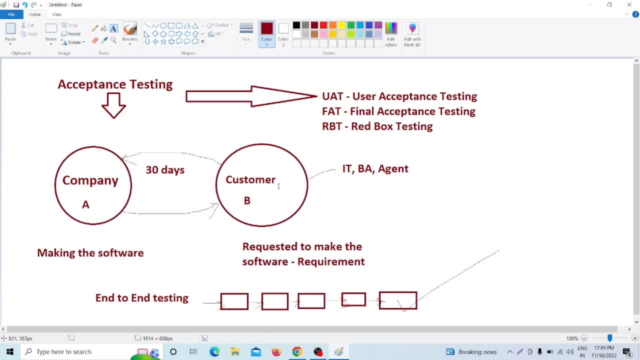 So they can test that application with that customer real time business scenario. So that is the one thing. That is the one thing. So, or we can say that. The fourth scenario: I can tell you that in that customer, So company A, has completed the software and they have given the software to the customer. 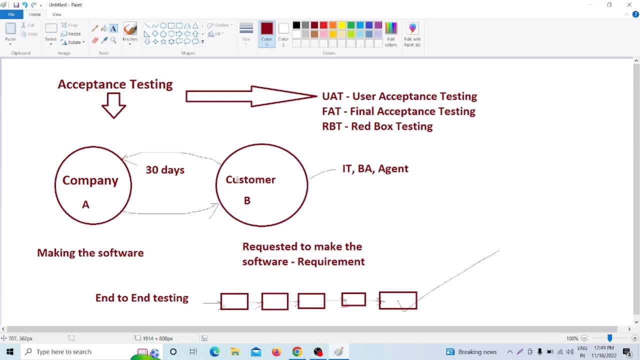 Now what we'll do. Customer will not take their software in that to their pocket. Okay, Obviously in that customer fields there are a lot of customer. So the customer is came to make their business. So that's why in that customer B they have lots of customer. 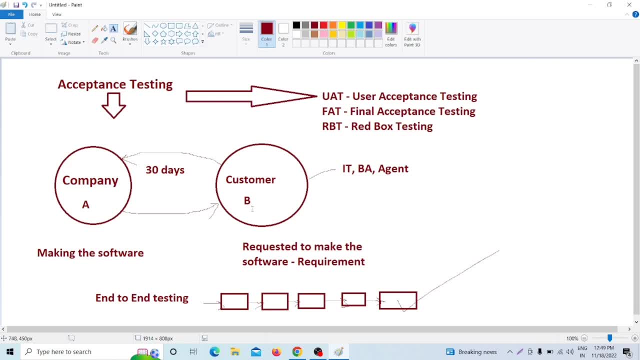 Okay, So what we'll do After giving the software to the customer B by the customer A, then customer B will circulate that software to their customer- Okay, Their stakeholder- and they will tell that: boss, can you please test that application by your real time business scenario, that which applications is developed by the company that is working perfectly fine, or not by their, by your real time business scenario? 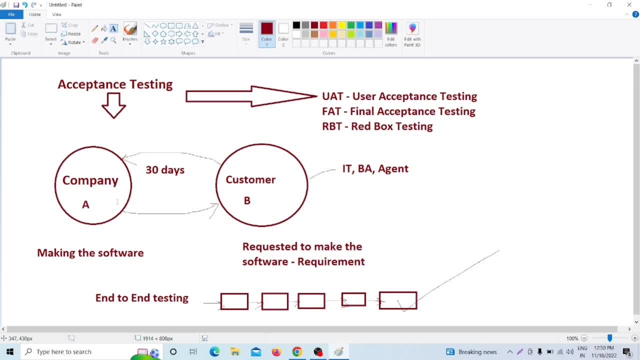 Right, That is the thing. So there are many ways we can check. So totally is depending upon on your views that how many ways you can test that acceptance testing. Okay, So now you guys are very much clear about that: What is acceptance testing and what are the way for that acceptance testing? 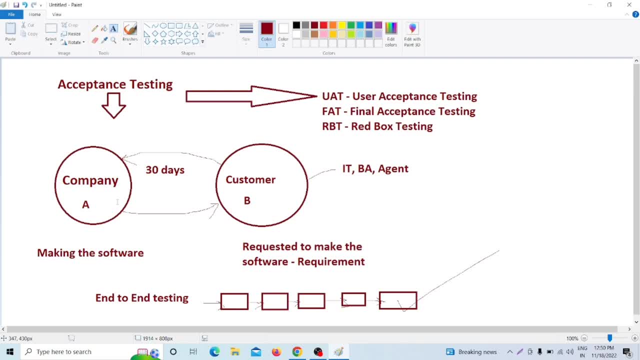 Okay Now. So what are the advantages of acceptance testing? Obviously there are some advantages. What is the advantages? Okay, So I can tell you that. the first advantage: that this acceptance testing helps the project team to know the further requirements from the user directly, as it involves the user for testing. 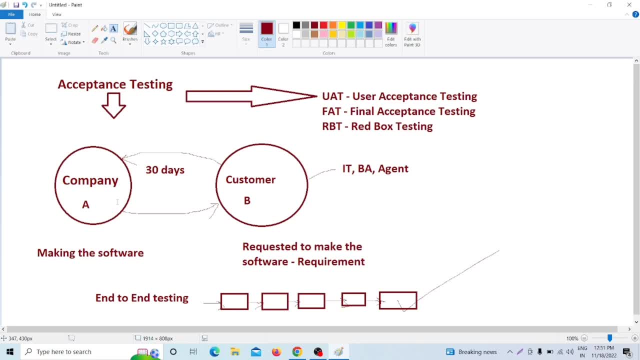 That is the most important point of the acceptance testing, or advantage of the acceptance testing. Okay, And second advantage, we can, I can say, tell you that it brings confidence and satisfaction To the client as they are directly involved in Thep темперances. 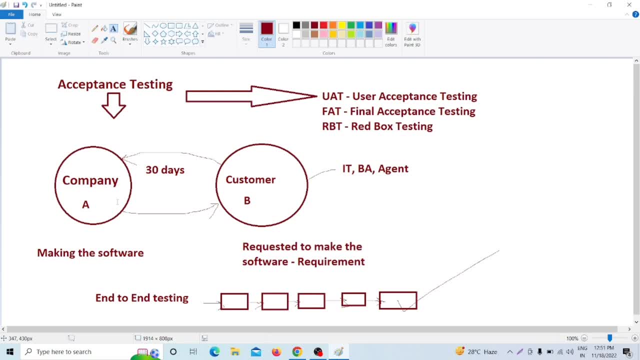 Okay, So obviously, as because accepted testing is totally done, done by the customer, order induced that, so customer will give some satisfaction. if the company is making the software as per the customer requirement, Then a customer is checking that arrogance team, that application, they will. 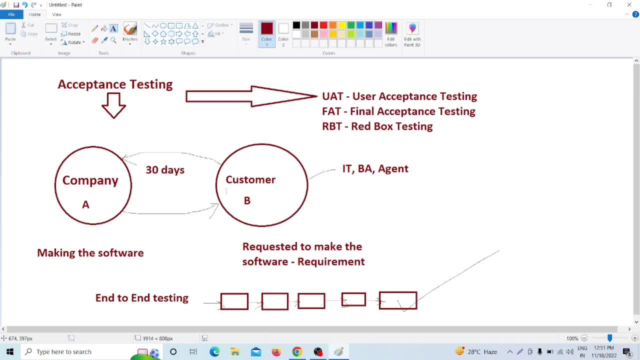 Keep some satisfaction, so they'll get some confidence that How, that yes, that yes, the software is working perfectly fine. okay, because the customer is directly involving the testing process. okay, or the third advantage: i can tell you that it is easier for the user to describe their requirement. okay, it is easier to the user to describe the. 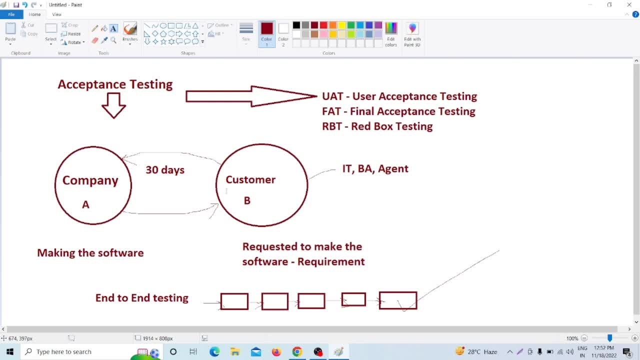 requirement. okay, and the fourth and the last point of the advantage, i can tell you that that acceptance testing is covers only the black box testing process. hence, the entire functionality of the product will be tested. so what is black box testing? a black box testing means we have to test. 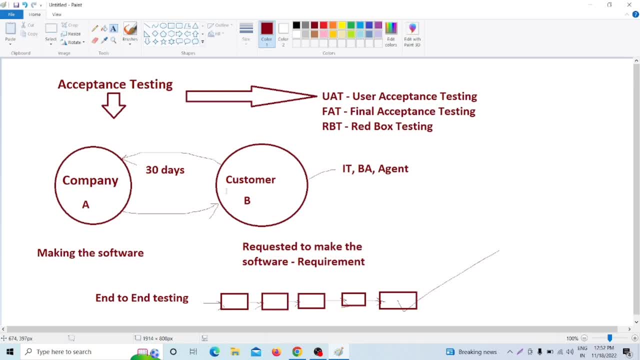 only the application but not knowing anything on the applications code or internal functionality or internal coding. we don't, we don't know that. what internal is? uh, what internal code is written by that? you the features. so we are checking only the input and we are getting the output as expected or not. 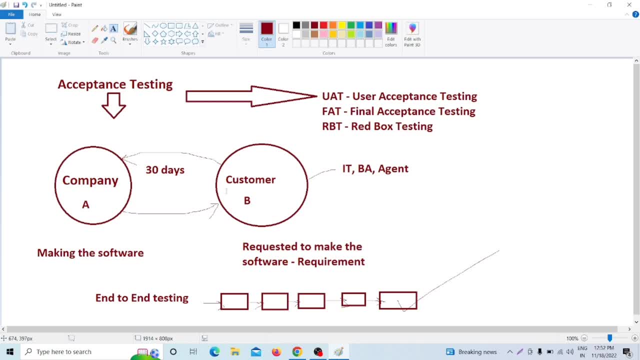 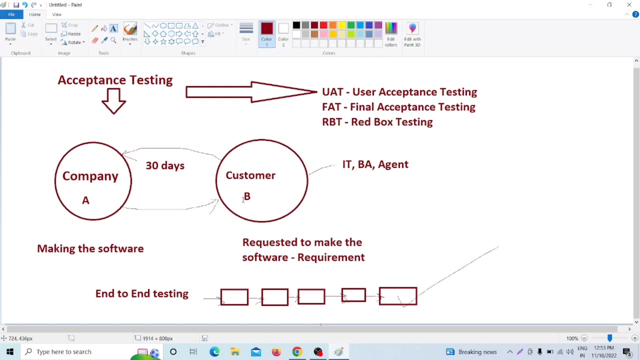 so, as acceptance testing is covers the black box testing, so we can tell that entire functionality of the product will be tested very carefully. so that is the most advantage of the acceptance testing. now, coming to the next one: is that disadvantage? what is the disadvantage? so disadvantage, the disadvantage. i can tell you that sometimes 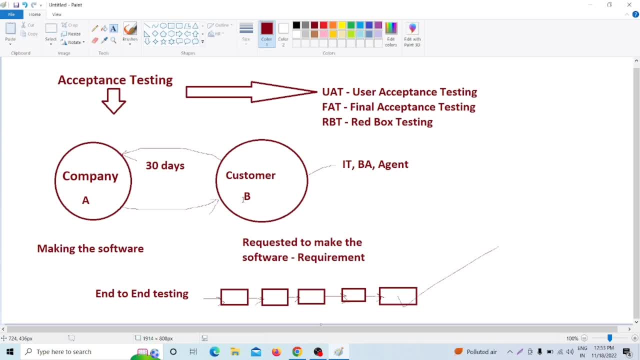 sometimes, sometimes user do not want to participate in the testing process. suppose the uh, the customer, the user, are very much busy with some other applications, sometimes maybe happen that they are not directly involving to that acceptance testing, so as because some of the requirements may be missed, right? so that is the one disadvantage and the second disadvantage? i can tell you that 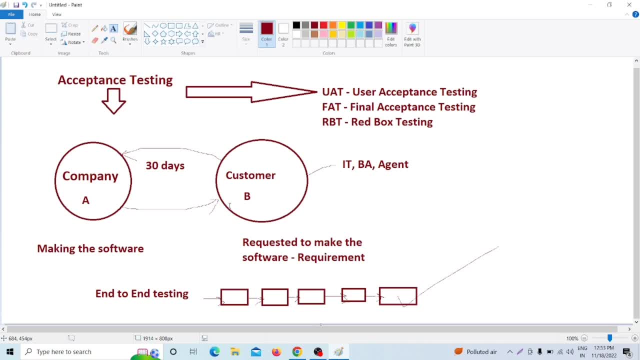 users should have basic knowledge about the product or applications. obviously, if the user don't have any basic knowledge, the application, so he will not able to test that. what is actually happening, what functionality is there? okay, so they have. they should have some basic knowledge of that application. okay, or third disadvantage: i can tell you that that development team is not. 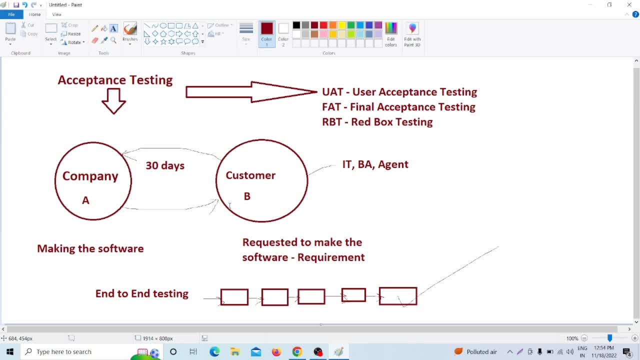 participated in the testing process. okay, development team will not participate in the testing process. development team only done, only make the software and they will hand over the software to the customer. now customer will take that responsibility to test the applications. okay, and the fourth disadvantage: that the feedback for the testing takes long. i mean 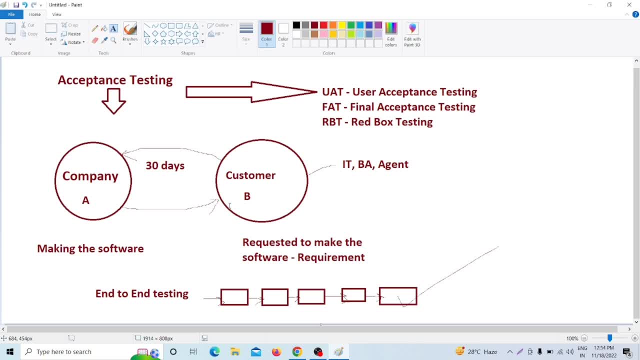 take long time as it involve many user and the opinions many may differ from one user to another user. obviously it will take some time because first the customer will test the application, then the customer- some customer, that customer has some different customer or different stakeholder. they will test.